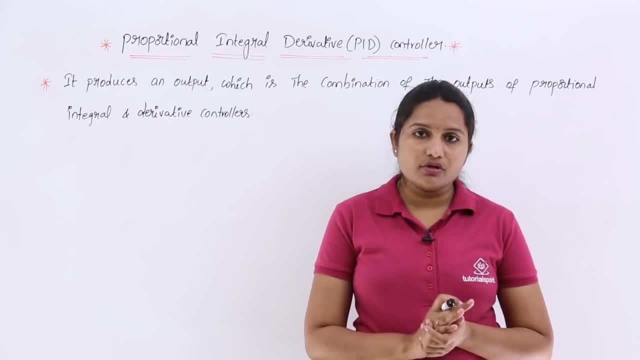 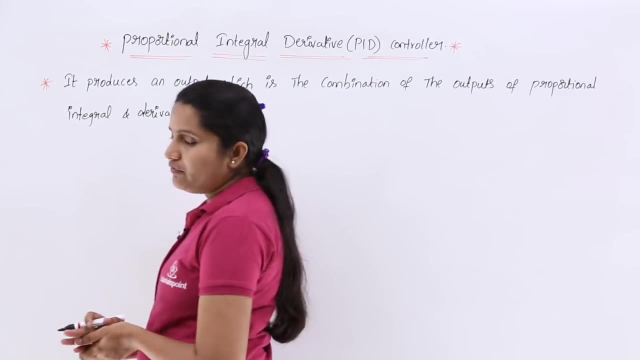 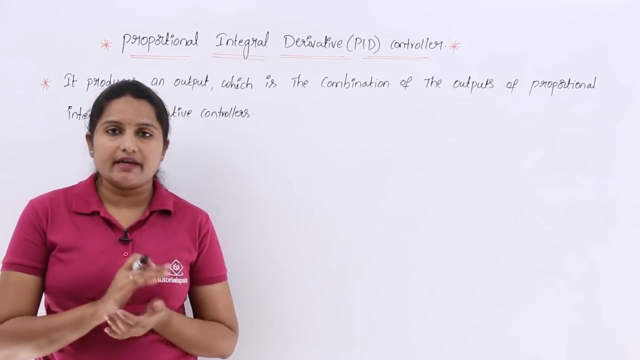 proportional integral differential controller, generally called as PID controller. So now we will see how we can analyze that controller, how we can sketch that block diagram of control system with PID controller. So now we will see for any controller from initial class of controllers. 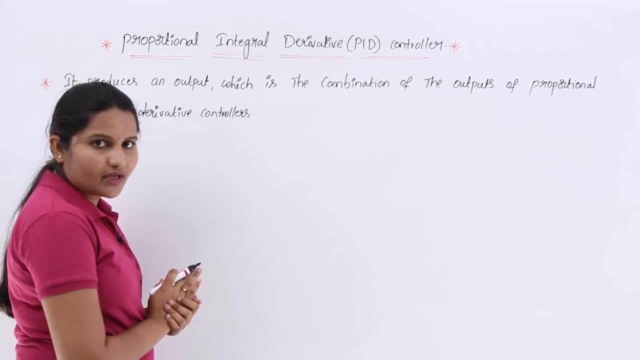 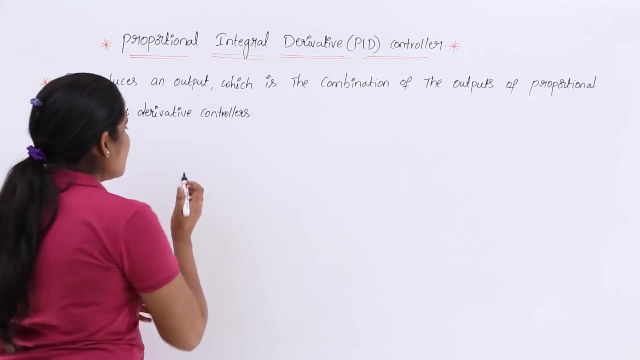 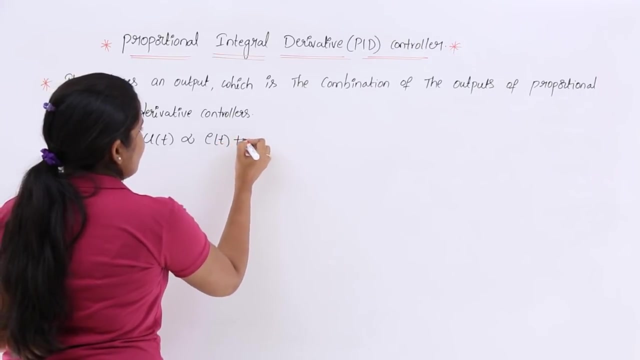 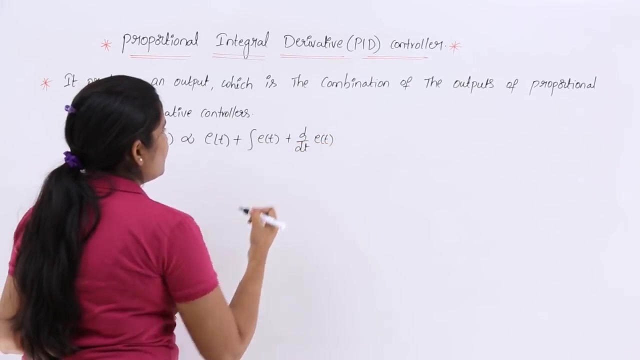 itself. we are discussing that the output of controller we are representing with u of t and input for any controller is error signal e of t. So your output must be proportional to proportional controller, integral controller and differential controller. So we need to combine all the controllers. 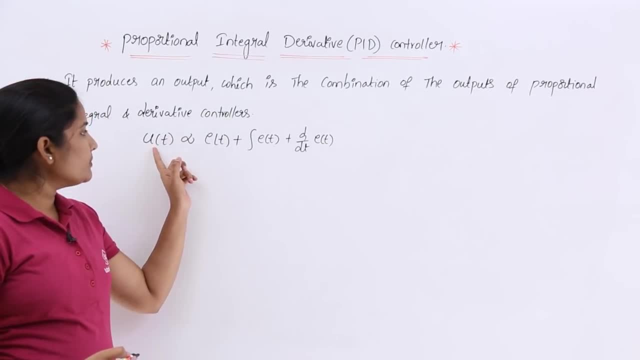 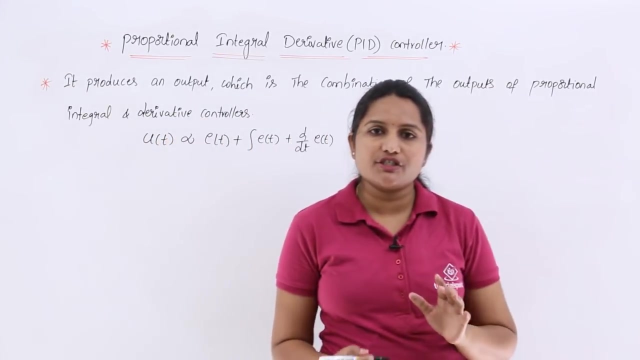 In case of proportional controller, the output must be proportional to error signal. In case of integral controller, the output must be proportional to integral of error signal. In case of differential controller, the output must be proportional to differentiation of error signal. but in case of proportional, integral differential controller, 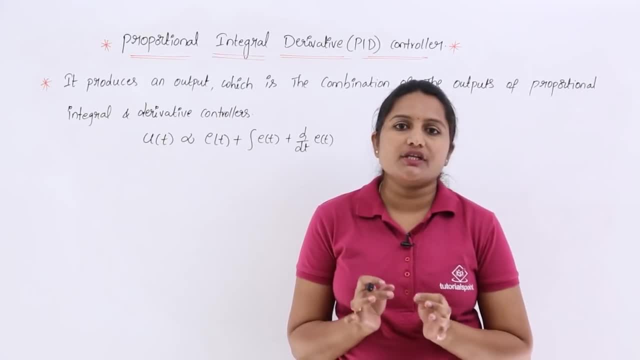 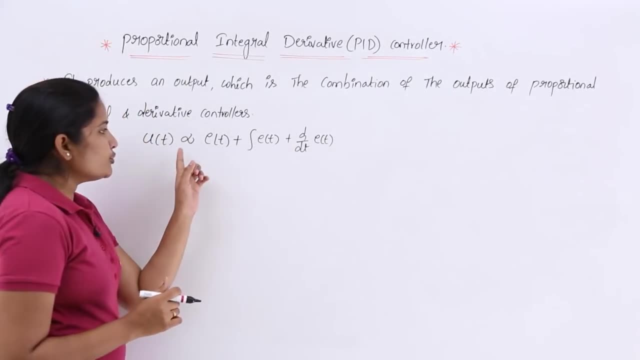 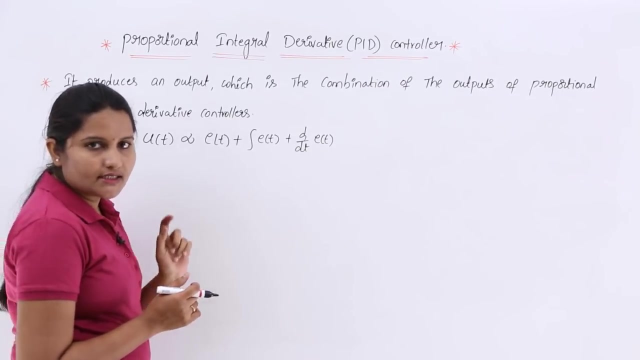 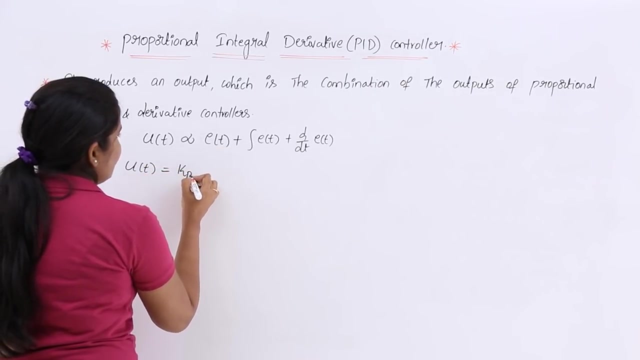 the output must be proportional to the combination of error signal, integral of error signal and differentiation of error signal. Now, to take out this proportionality, I need to use coefficients here, I need to use constants here. So u of t is equal into to equate a of t. I am writing kp. 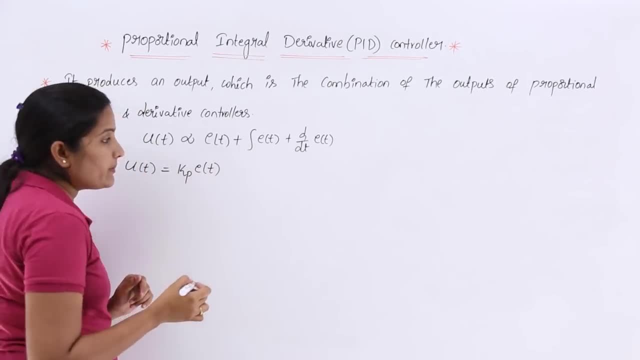 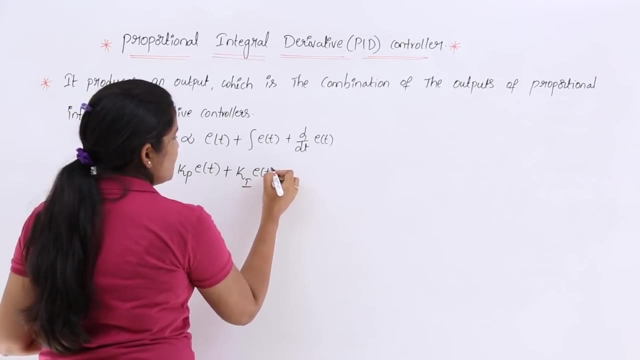 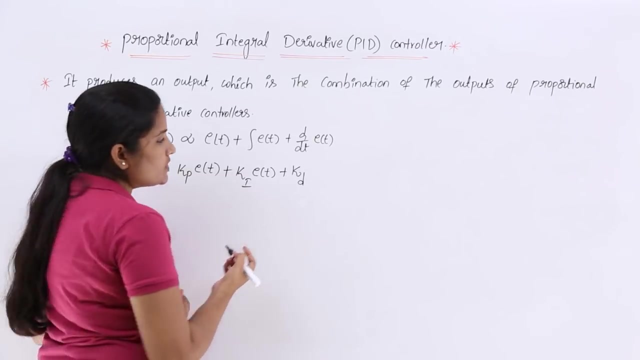 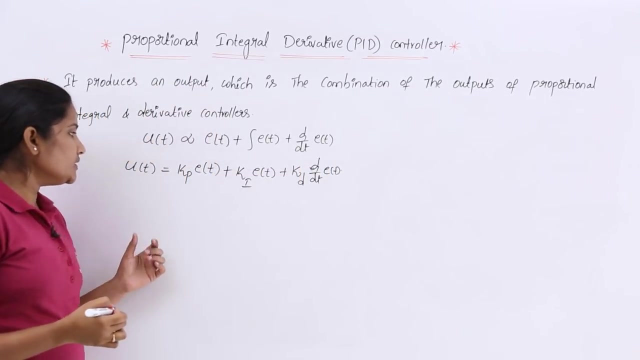 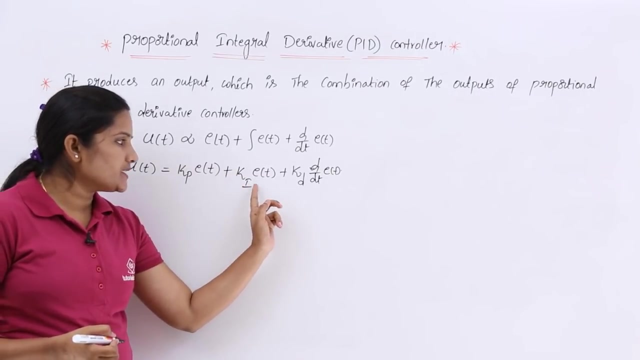 because that is proportional controller part. and to equate integration part. so I am using ki into a of t. So, similarly, to equate the differentiation part, I am writing that constant as kd, so which is nothing but differential constant. So this will be your output of PID controller, where u of t, equivalent to kp, into a of t. 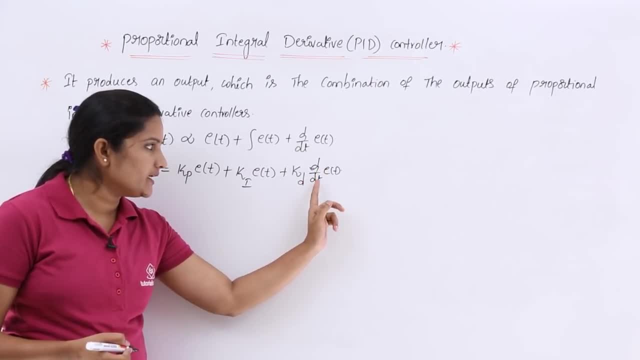 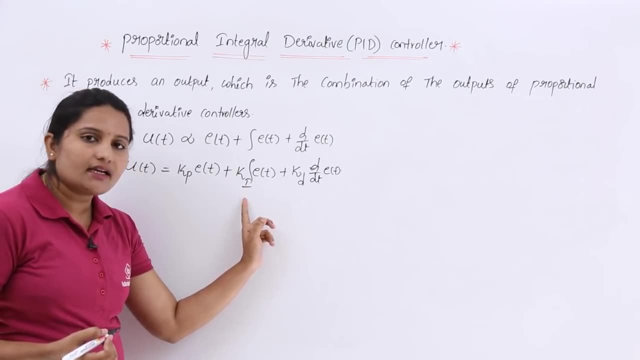 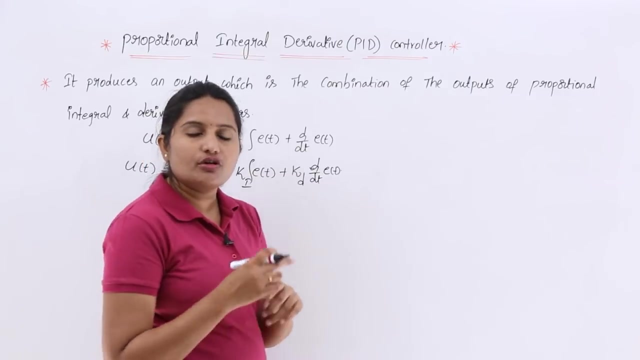 plus ki into a of t, plus kd into d, by dt of a of t, this is integral a of t. So now, where kp is the proportionality constant, ki is the integral constant and kd is the differentiation constant. Now the thing is, we want to draw a. 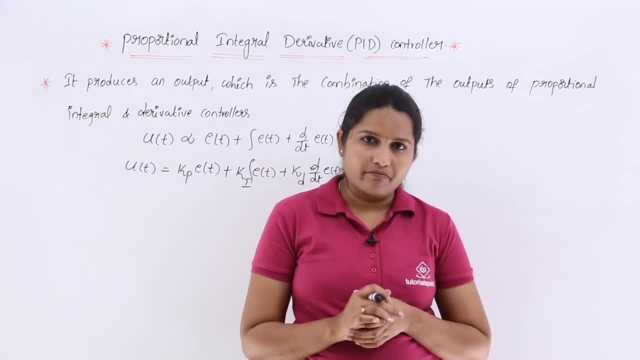 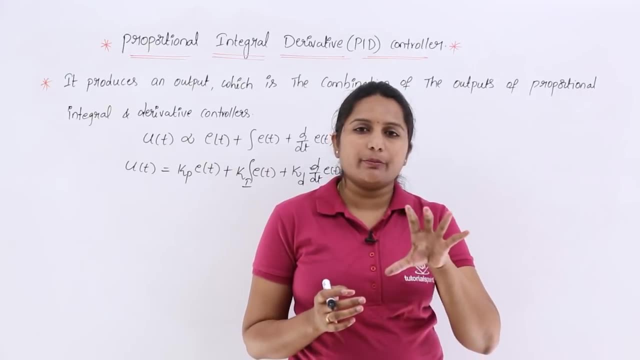 block. So we want to draw a block. So we want to draw a block. So we want to draw a block. Block diagram of the control system with PID controller In control system. block diagrams, if you want to represent any controller. how we can represent means we can represent with. 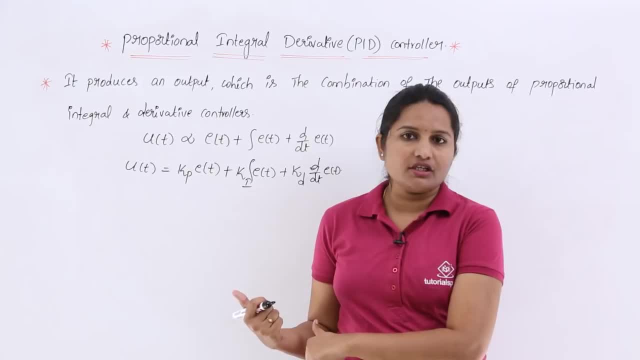 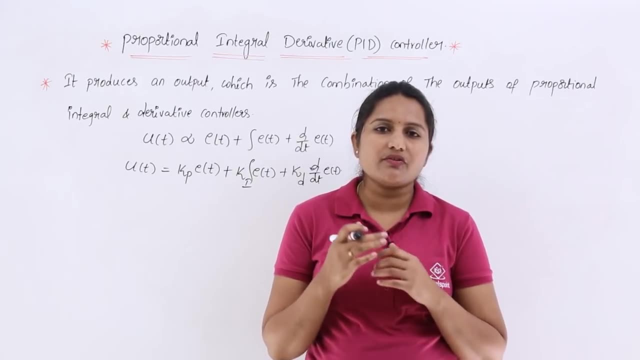 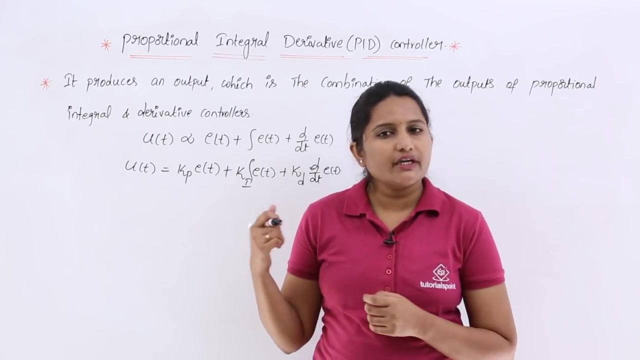 transfer function. So we need a transfer function of PID controller. now We are having output and input in the form of time. that means in terms of time. if you need transfer function, then you need to convert this. So you need to convert this. So you need to convert this. So you need to convert. 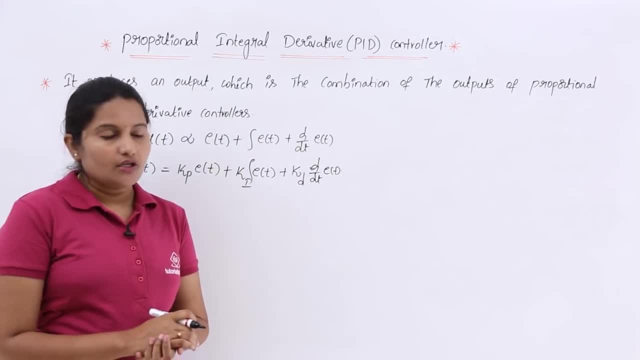 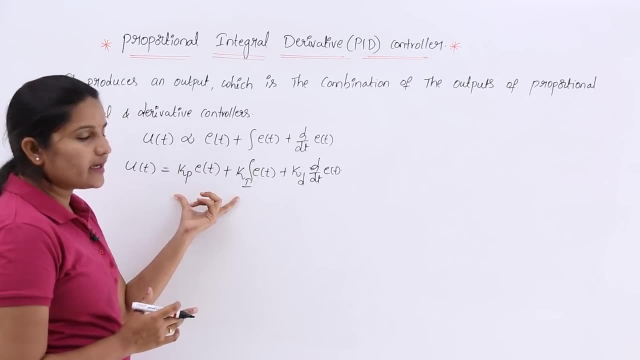 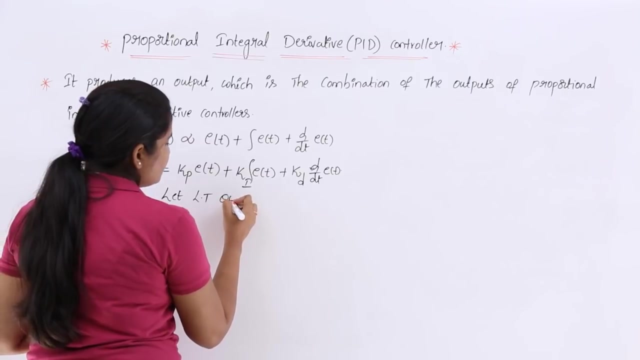 this time domain into frequency domain or s domain. So that is why, to calculate transfer function further, I am going to convert this time domain into s domain by taking Laplace transform. So let Laplace transform on both sides. On both sides, if I am taking Laplace transform, then u of t is: 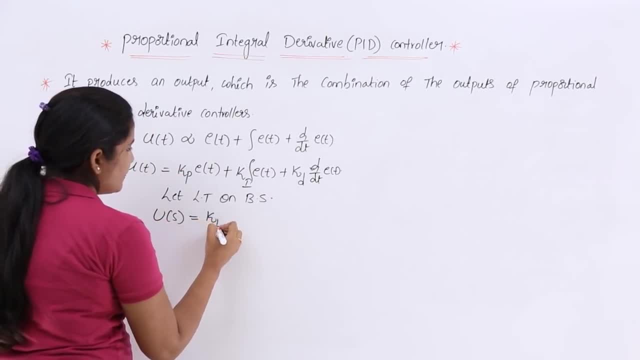 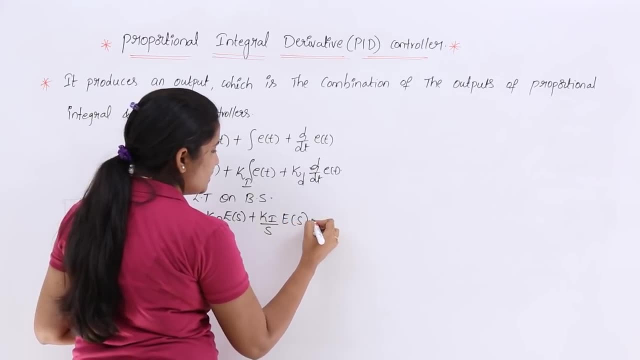 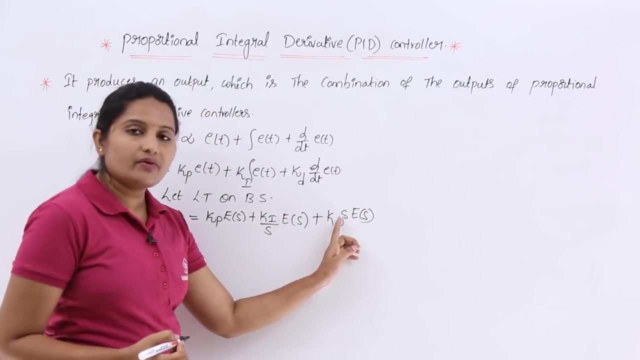 equivalent to u of s. This is equivalent to kp into e of s. This ki by s into e of s. because integration, like that kd into s into e of s. If differentiation is there, Laplace transform will give you multiplication in s. If integration is there, Laplace transform. 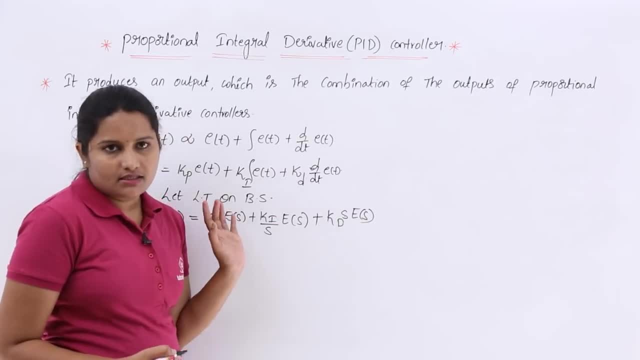 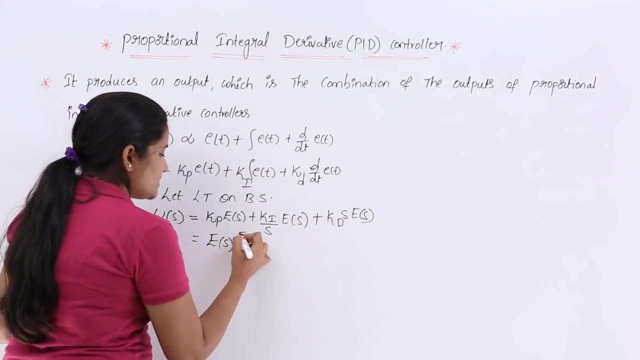 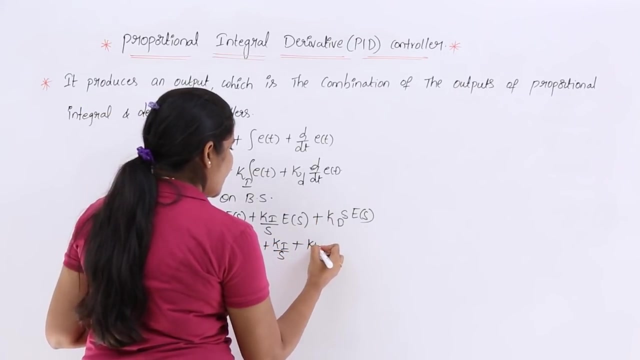 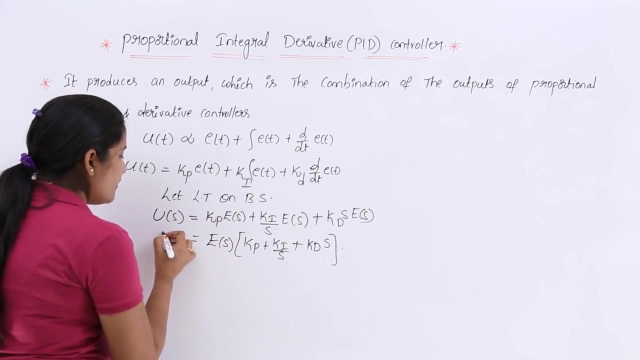 will give you denominator s. So this is your u of s. Now I am taking common of e of s here. E of s into kp plus E of s is equal to kp plus ki by s plus kd into s. So now here u of s is equivalent to e of s into k p plus ki by s, kd into s. 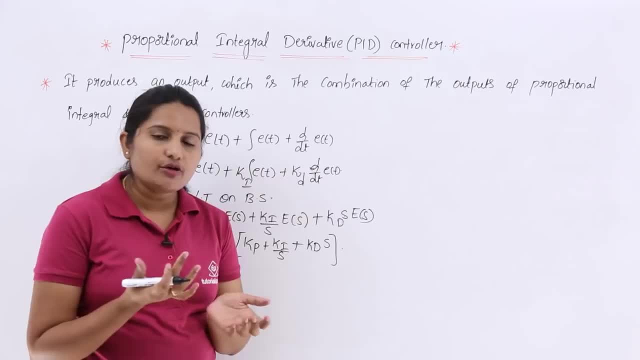 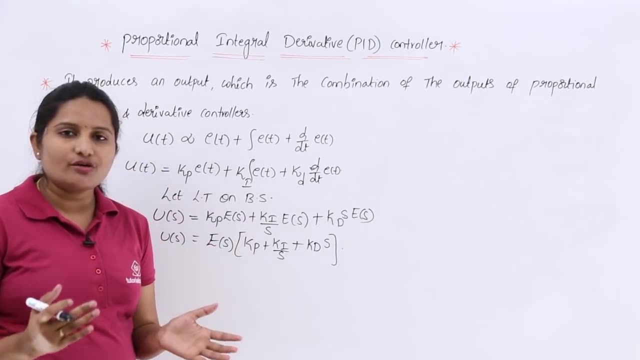 This is what you are getting after taking Laplace transform. Why you take in Laplace transform To derive the transfer function. How will get transfer function? The definition of transfer function for any system is the expression of the transfer function. So the definition of the 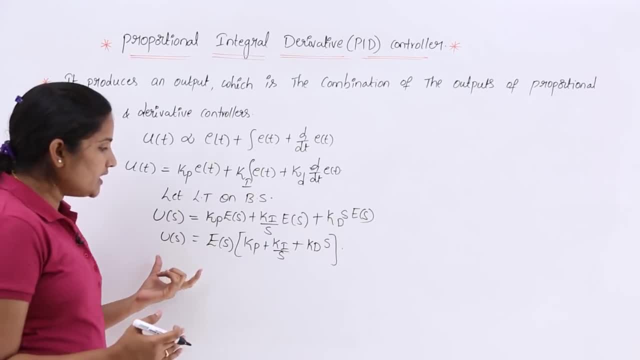 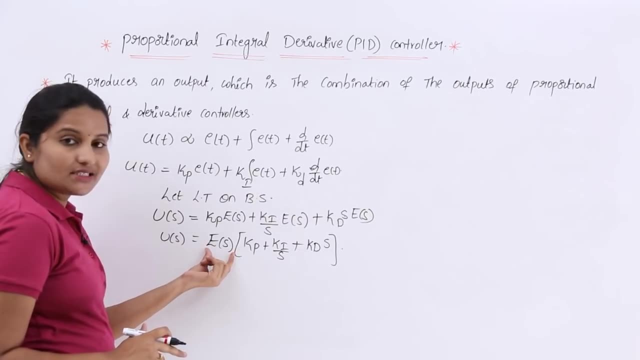 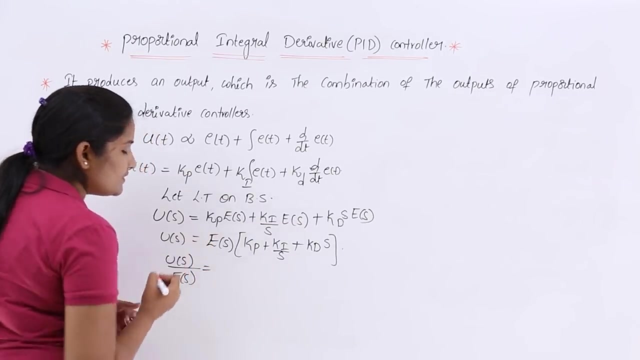 is output transform by input transform. So here for a controller, output is U of t, input is error signal. Output transform means U of s, input transform means E of s. So by considering U of s by E of s, then you are going to get the transfer function of the. 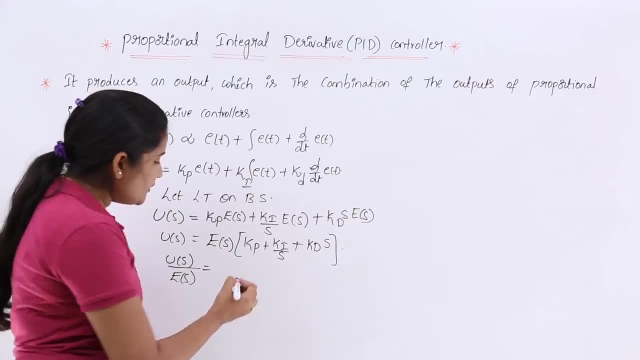 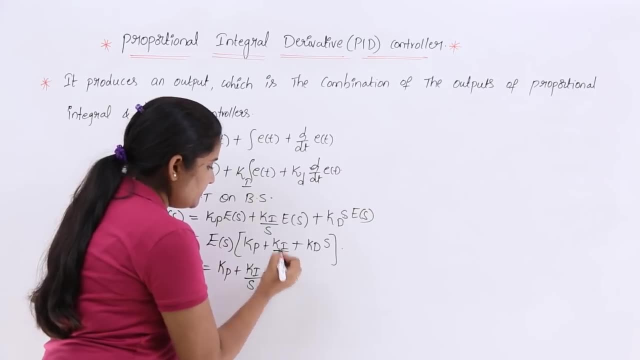 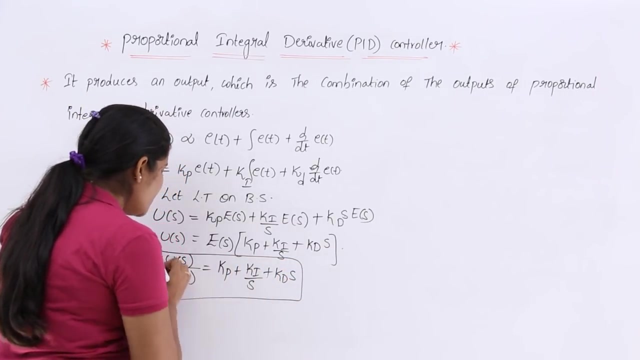 system. So U of s by E of s is equivalent to K p plus K i by s plus K d into s. This is what we are getting. So this is the transfer function of PID controller. if you want any simplification for this, you. 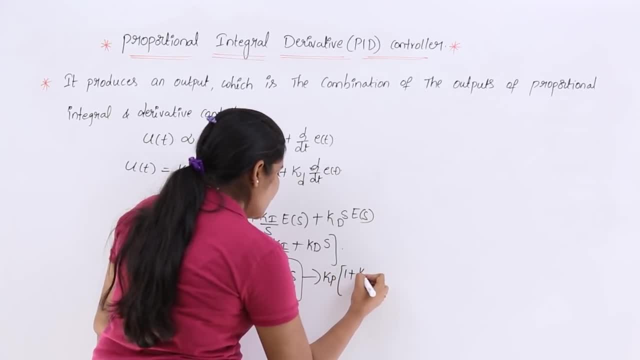 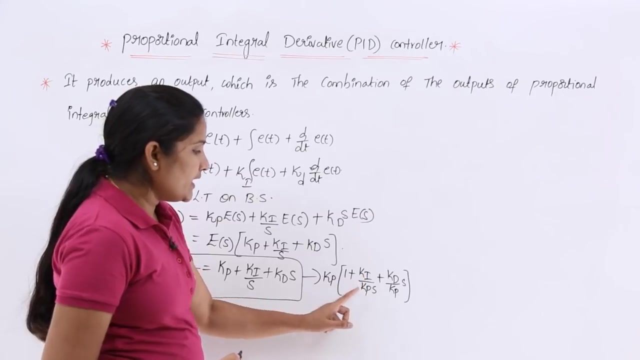 just take common of K p 1 plus K i by K p, E by 1, K p by E of s is from K d to K p plus K d into S And you can write a controller by primary into S plus KD by KP into S. So you just consider KI by KP as I am just considering. 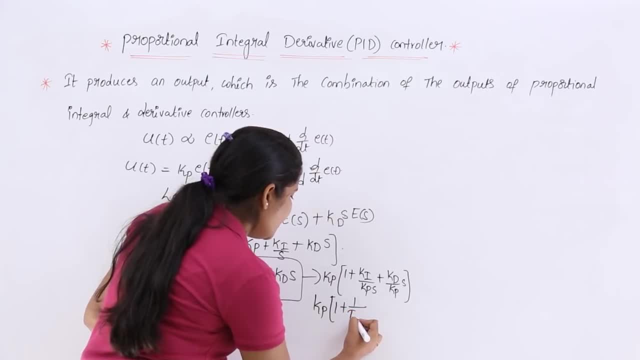 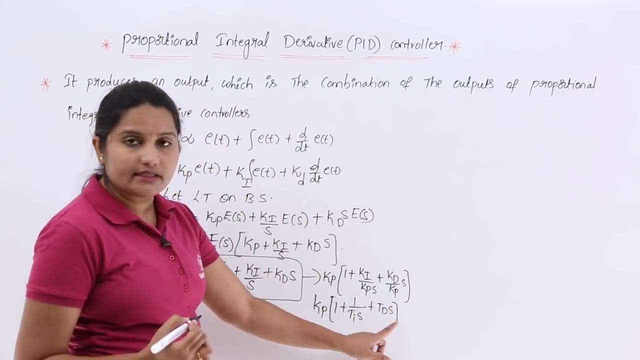 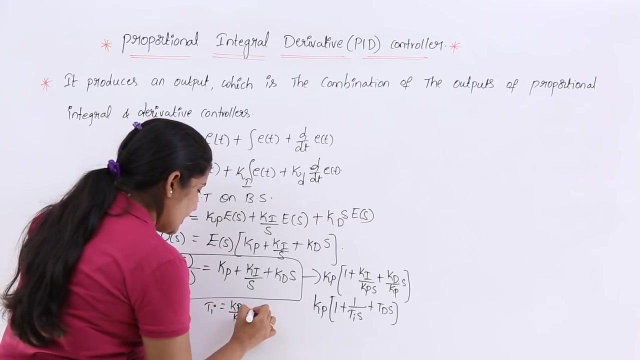 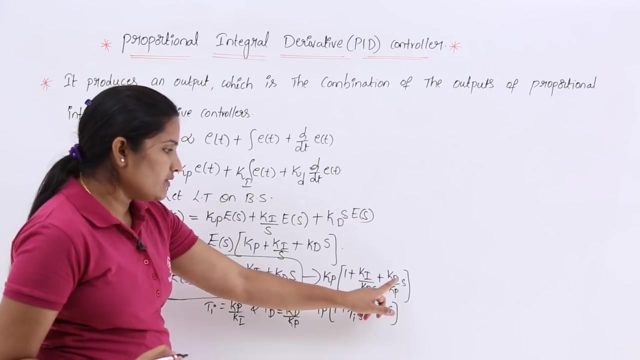 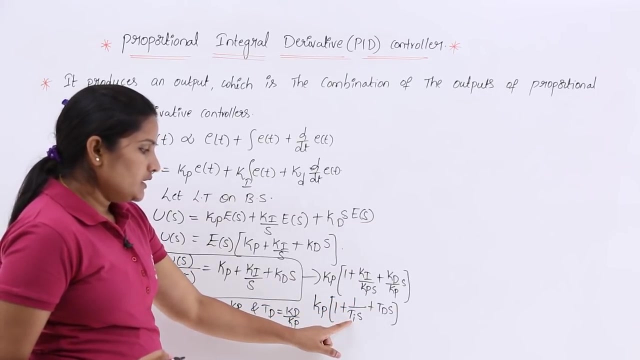 like this: You can see 1 plus 1 by TI into S plus TD into S. I am just considering like this: Where TI is equivalent to KP by KI and TD is equivalent to KD by KP, You can see: TD is equivalent to KD by KP, TI is equivalent to KP by KI If you substitute KP by KI here. 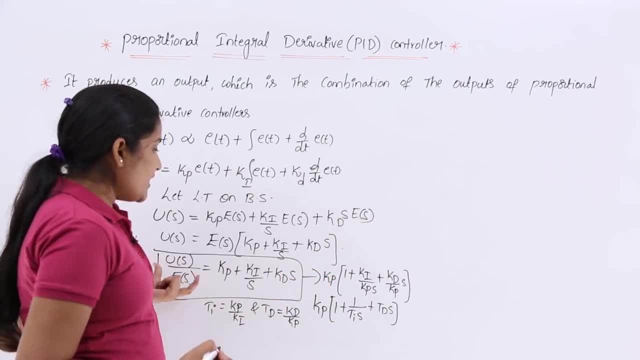 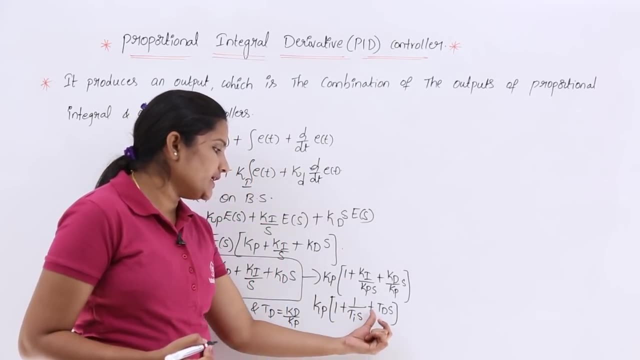 you will get this same. So the transfer function of PID controller is just like this And the transfer function of PID controller is just like this. So you is equivalent to Kp into 1 plus 1, by Tis plus Td into S. Now, with this, I am going to draw the block. 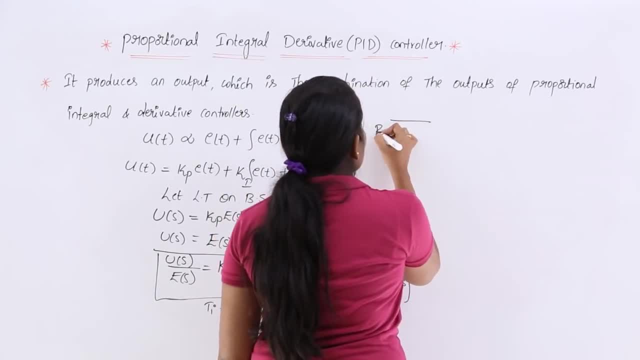 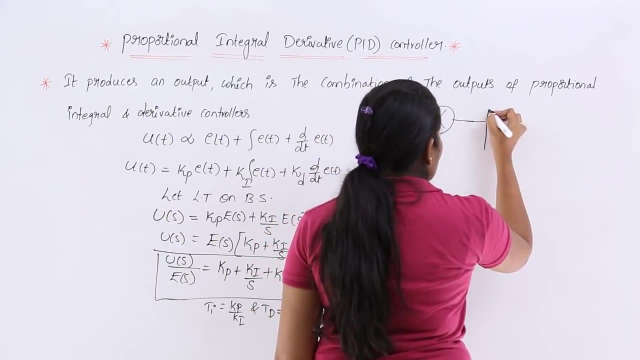 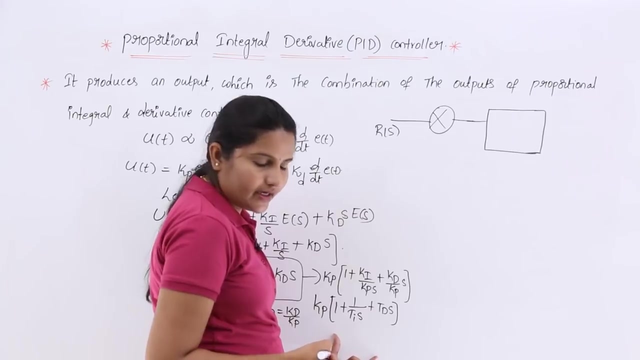 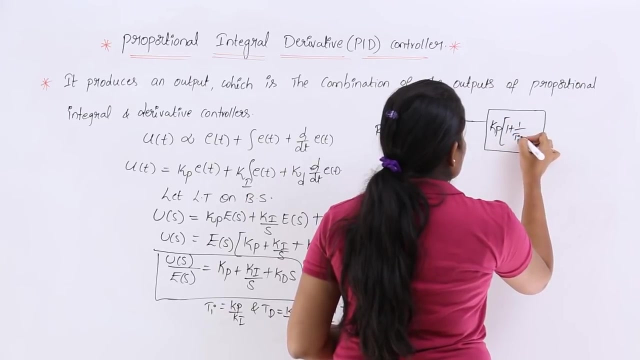 diagram now. So block diagram of control system will contains the input transform first and after that. if I want to add this PID controller, in what sense I can add means by adding transfer function. we can say we are adding the PID controller. this is the transfer function: Kp into 1 plus 1 by Tis. 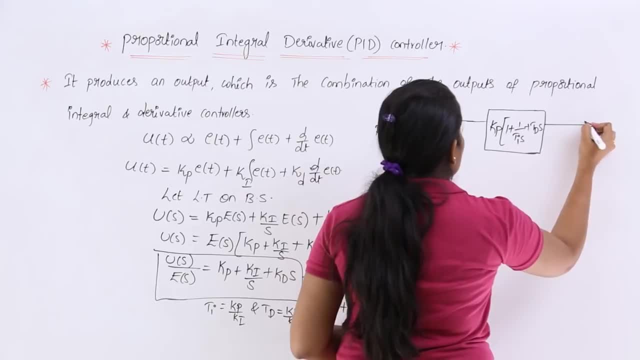 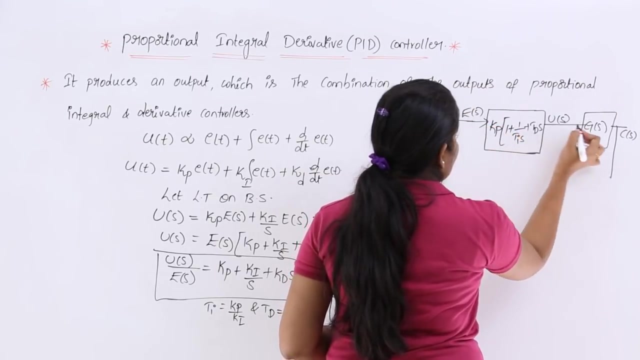 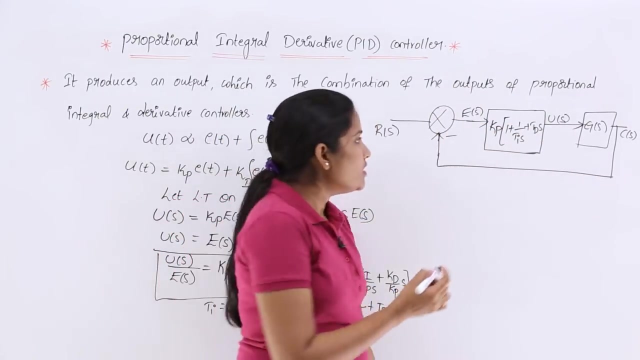 plus Td into S, So input is E of S, output is U of S. So here I am taking gain, So this is C of S output, and negative feedback, So this is U of S. So this is your control system with the PID controller. So up to here, this is PID controller. 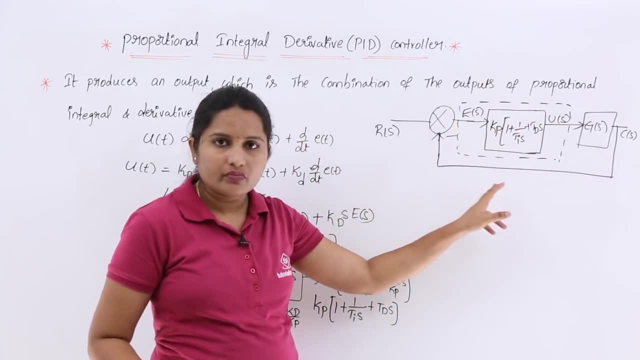 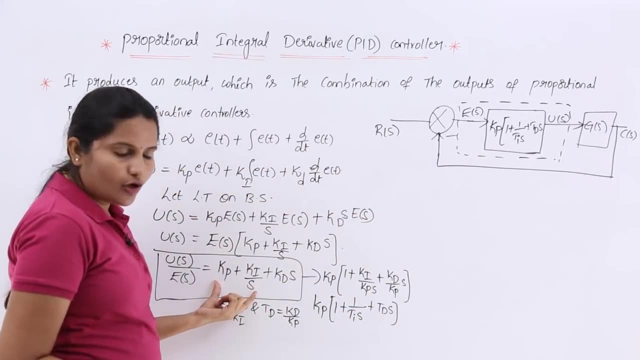 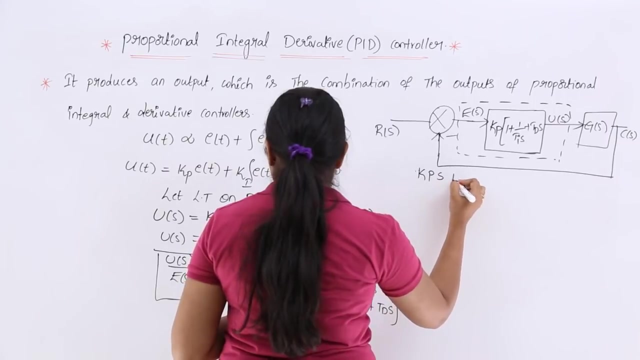 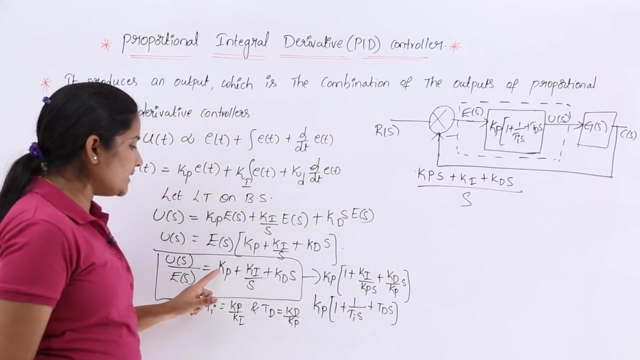 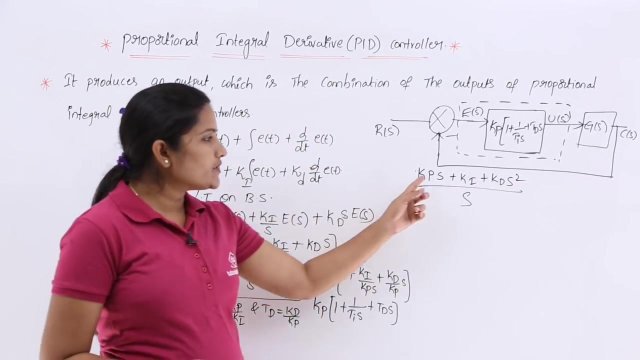 This is your PID controller. So here, if you observe this transfer function, I can write this transfer function as Kp into S plus Ki plus Kd into S divided by S. I am just cross multiplying and writing this S square, not S, If you observe these two. 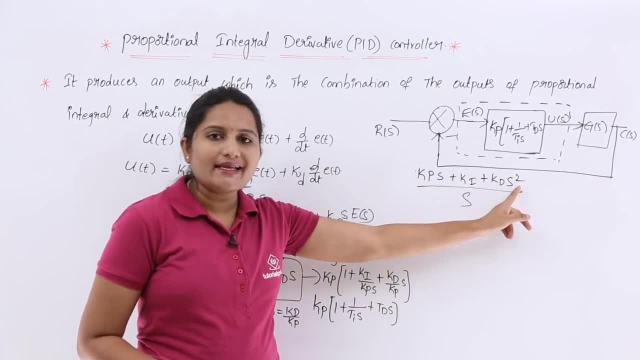 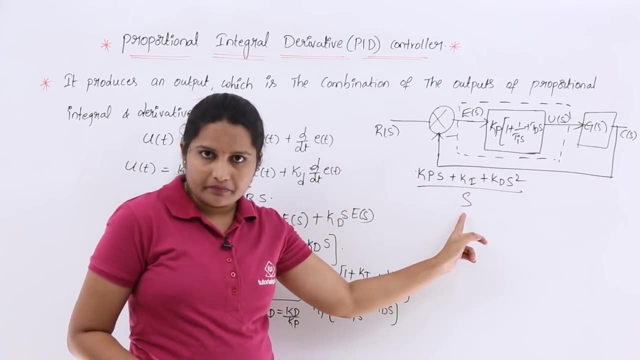 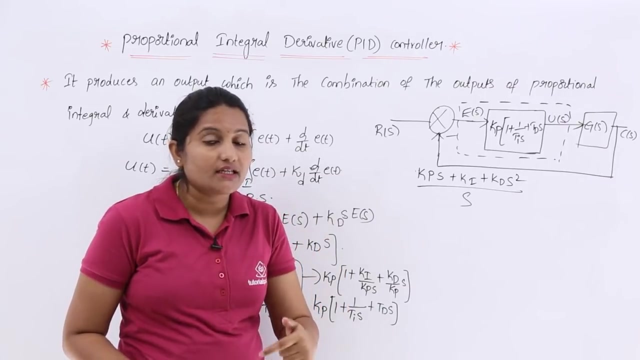 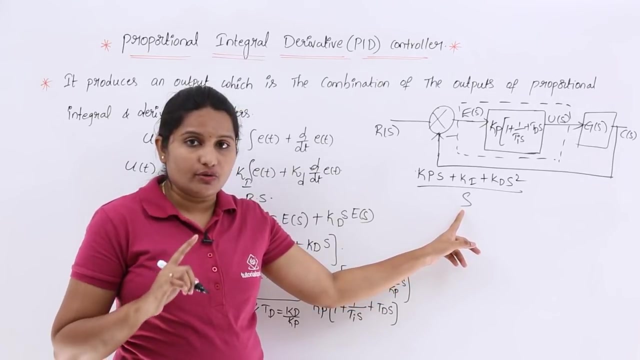 it introduces two S terms in numerator. that means two zeros are introduced and coming to denominator one S term is there. It introducing one S term in denominator, that means it increasing the type, So it is increasing a pole at zero. It introducing pole at zero. You can see the transfer function of this. 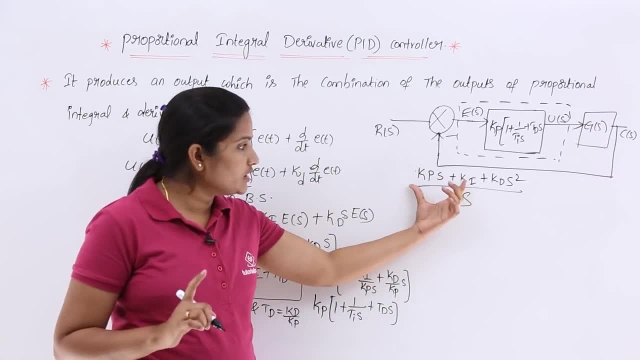 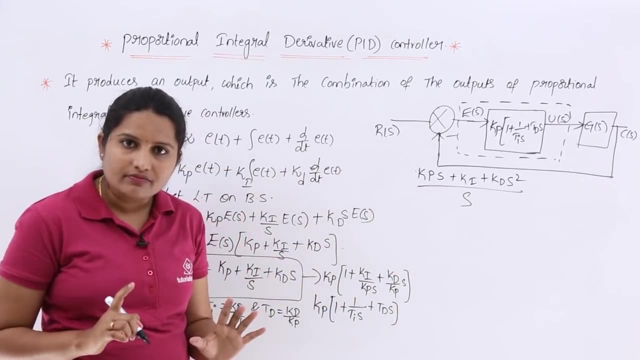 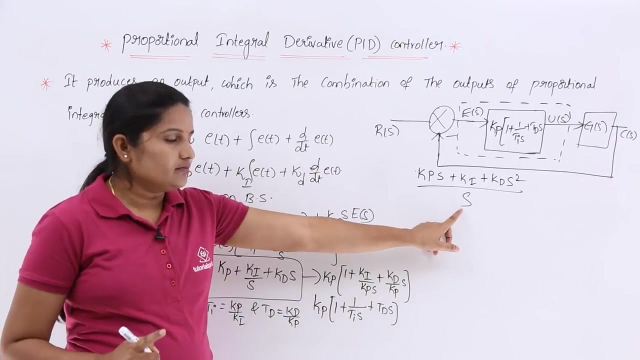 I am just simplified, this controller's transfer function. So by this transfer function you can say: in denominator S term is there. That means the type number is going to increase. That means we are introducing a pole at origin. The meaning of denominator S means we are introducing a pole at origin. 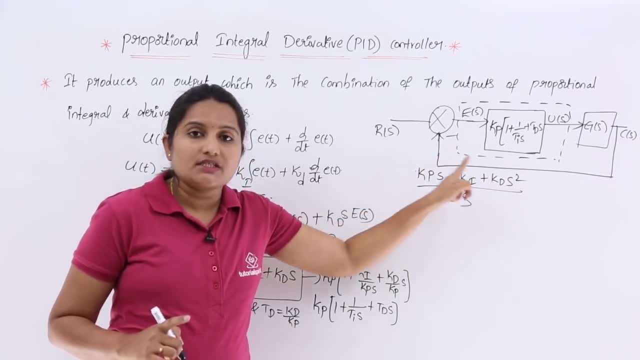 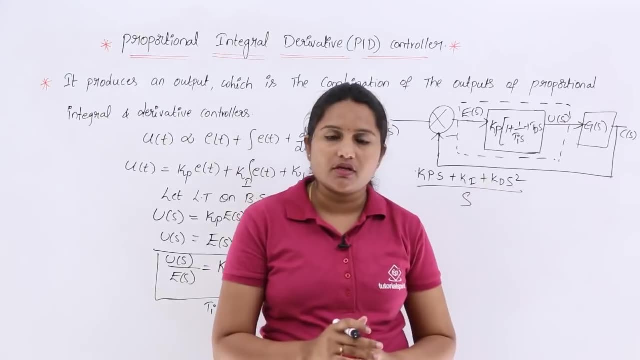 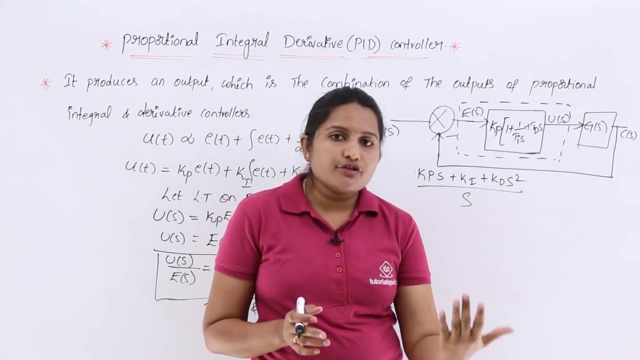 And we are having two S terms in numerator. Two S terms in numerator One is S term, one is S square term. Two different S terms. By that we will get two coefficients. that means two zeros. So we are introducing two zeros. We are introducing one pole at origin. 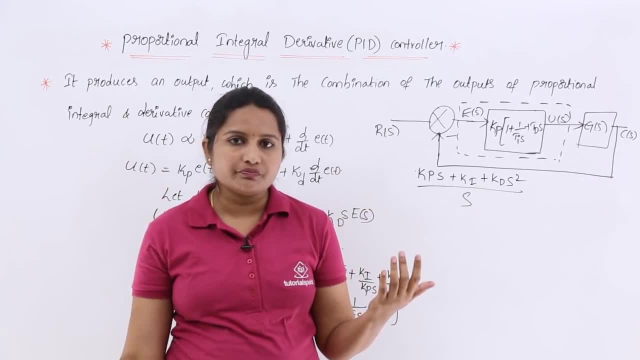 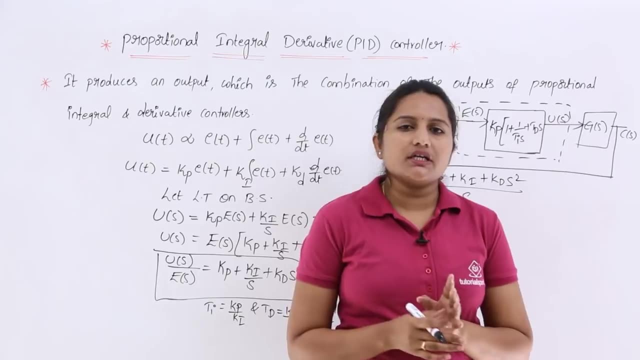 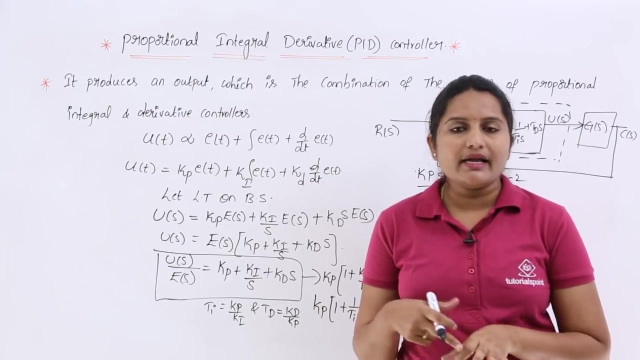 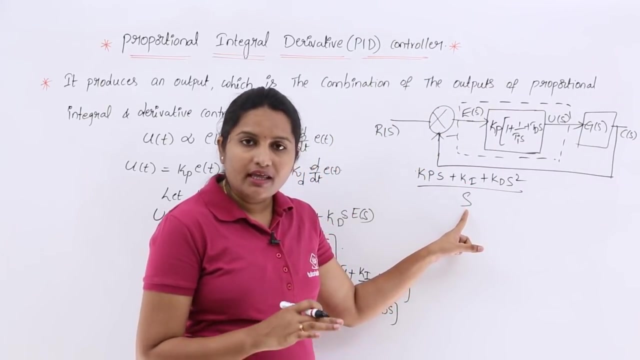 One zero can compensate one pole. another 0 will increase the stability of the system. Generally, PID controller is used to increase the stability as well as to decrease the study state error by increasing the type number of the system. By introducing pole at origin, you can increase the type number of the. 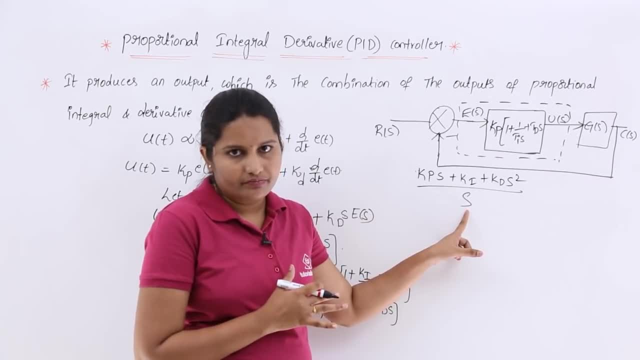 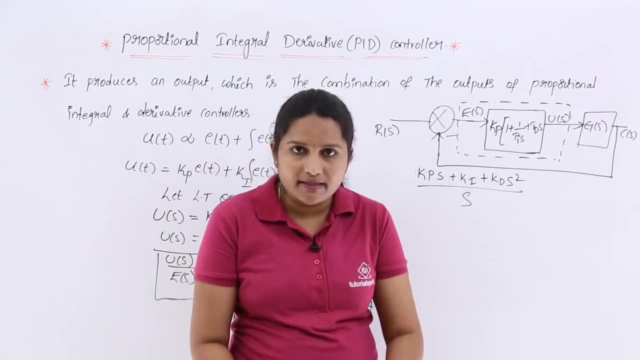 system that implies study state error will be decreased By introducing the 0s in numerator. by increasing the 0s you can increase the stability of the system. Previously also in PD controller, PI controller also, we introduced one 0 at numerator. but that 0 is going to.